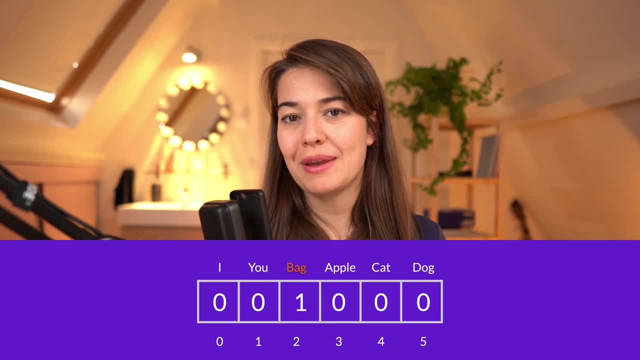 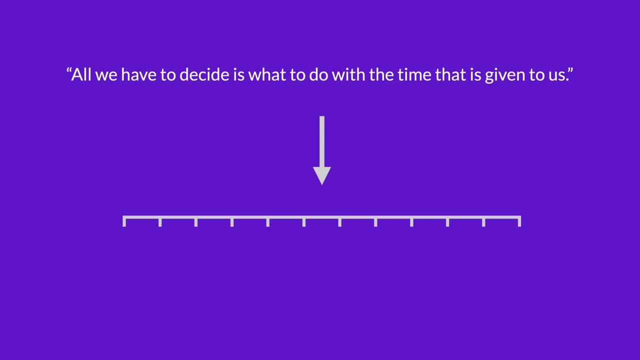 sparse vector and it is not the most efficient use of space. So let's see how else we can achieve this Text representation. Count-based representation techniques generally try to squeeze a whole sentence into just one vector. There are a bunch of different approaches under the umbrella of 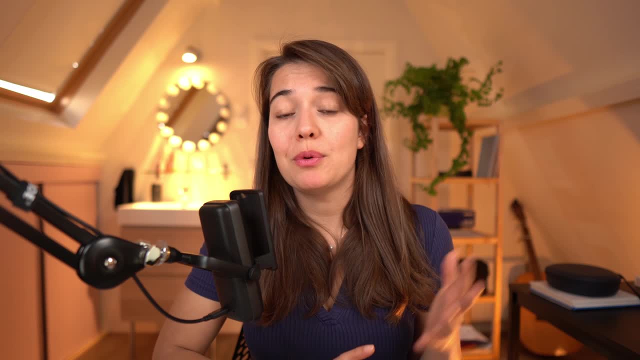 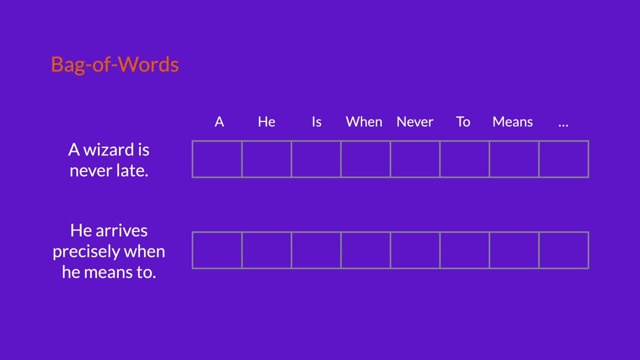 count-based representation techniques. Some of them are, for example, bag of words In bag of words. what you do is you do not think about the order of the words in a sentence, You just look at how many times each word occurs and you create a vector to represent this. Then you have the 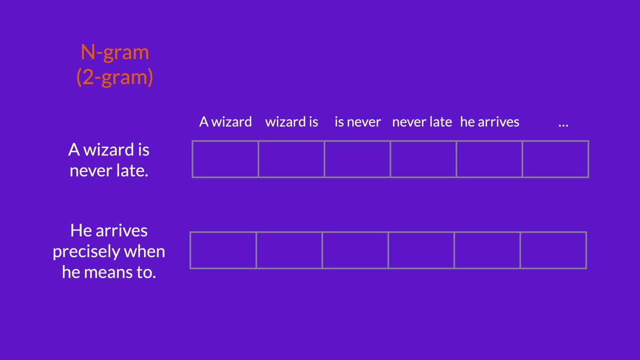 engram approach. that is quite similar to the bag of words approach. You just look at how many times each word occurs and you create a vector to represent this. Then you have the tf-idf approach, but this time you do not just take one word, but you make groups of n words and count their occurrence in. 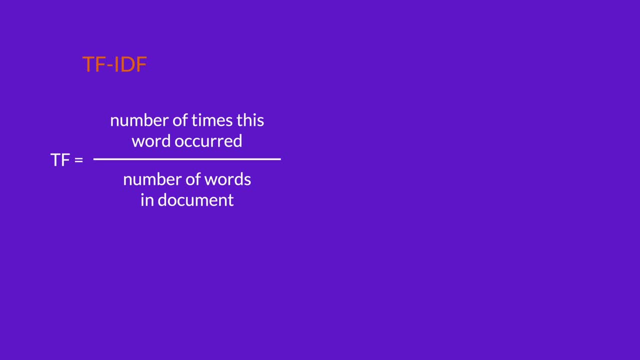 a sentence. And then you have the tf-idf approach, where you keep track of how many times a word occurs in a document, or also called sentence, and how many times this word occurs in other documents or sentences throughout the training data, And this way it is aiming to differentiate the words. 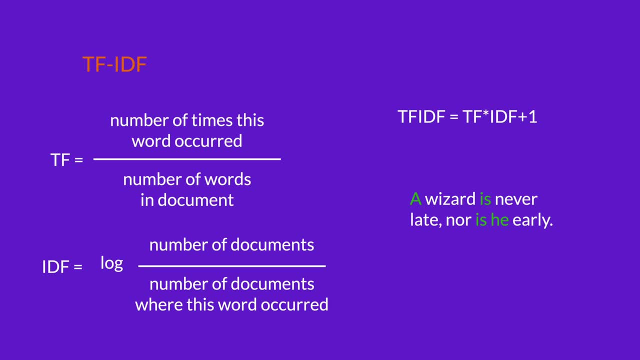 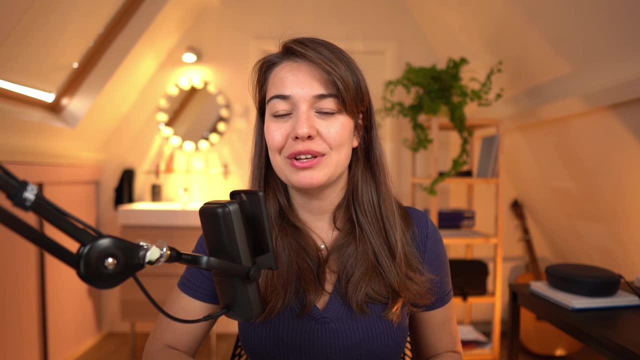 that are just commonly used, like d, of, and, and the words that are used in the training data And the words that are specifically important for a certain sentence or document. These approaches, even though they've been really helpful in the NLP area for years, have some serious shortcomings. 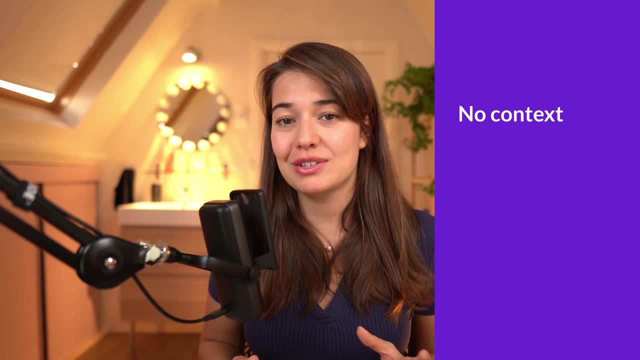 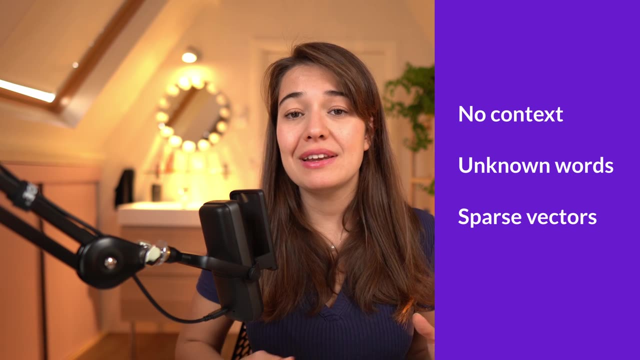 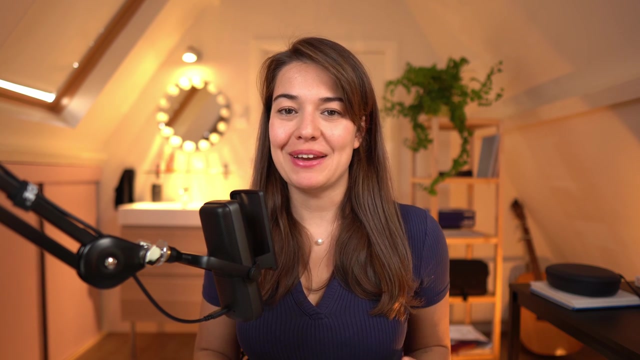 So, for example, they do not take any context into account. Furthermore, they cannot deal with words that they did not see in the training examples And, lastly, the embeddings that they produce are very sparse, so they are not the most efficient use of space. Now let's talk about embeddings. 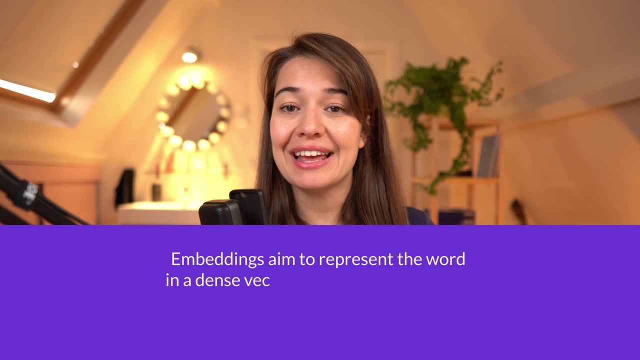 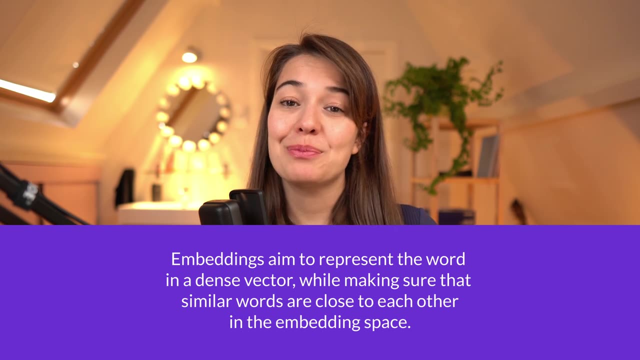 The goal of making word embeddings is to reduce the number of words that are used in the training data. The goal is to represent the word in a dense vector, while making sure that similar words are close to each other in the embedding space. Okay, let's break that down. What does a dense vector 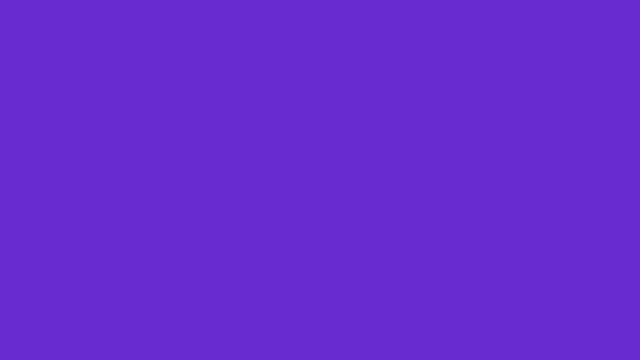 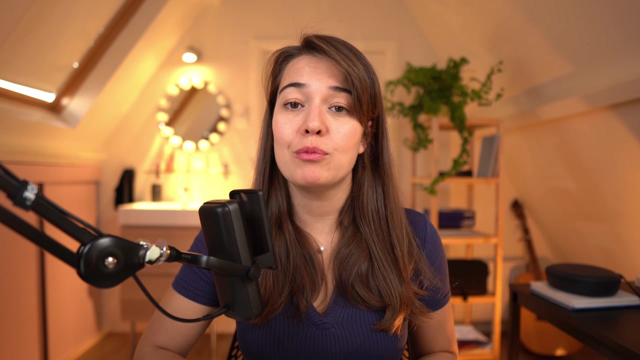 mean Having a dense vector, means that the vector representing the word does not mostly consist of zeros And typically the embedding of the word has fewer dimensions than the number of words that you have in your vocabulary. Okay, and what does it mean for words to be similar? So similar words are. 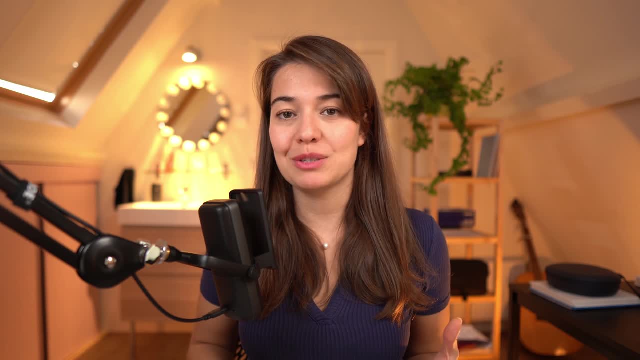 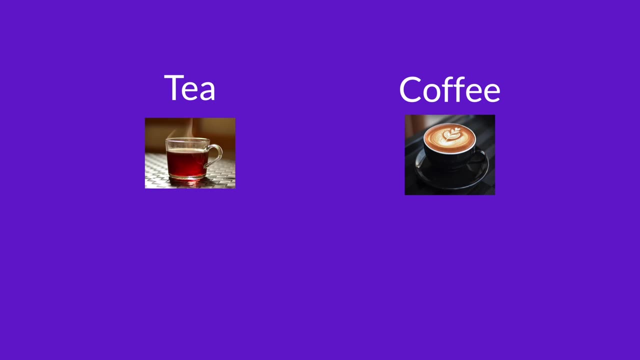 words that are used in similar or similar words, So the word embeddings are used in similar or similar words. You would see them being used around same words. So, for example, for words tea and coffee, you can think of them as similar words, because you would always see them being used around the other words. 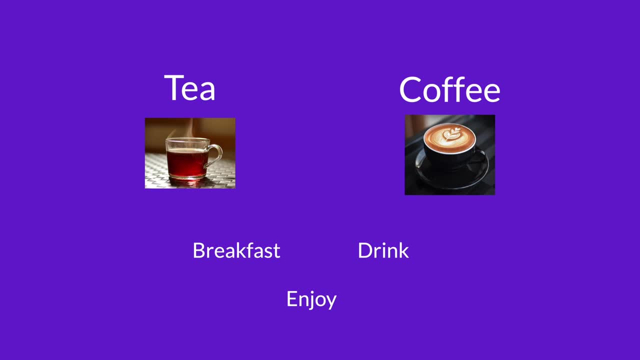 such as breakfast, drink or enjoy, Whereas the word pea, which is a legume, and tea are not really similar words, even though they are spelled really similarly, because they are used in vastly different contexts. So once we have the embeddings of these words, we can use them in different contexts. So let's start with the embeddings. 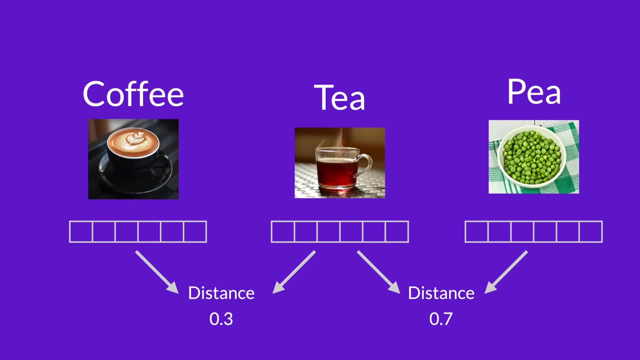 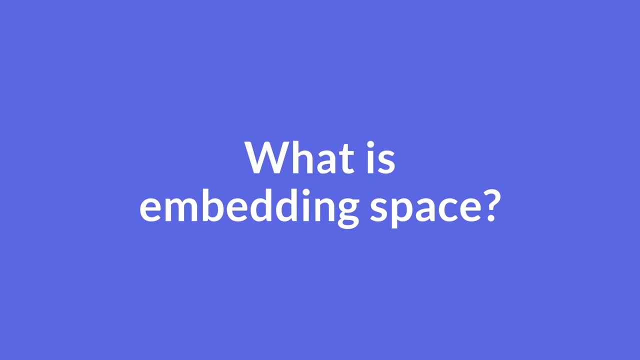 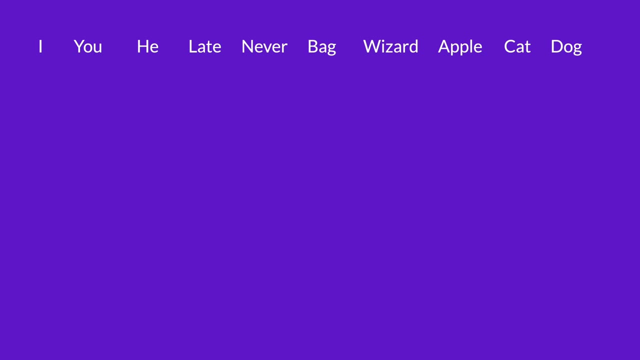 words, we would expect the vectors of the words t and coffee to be much closer to each other than t and p. and lastly, what is embedding space? embedding space is where your embedded data lives. so let's say you have 10 different data points and their mathematical embedding, one-dimensional embedding. 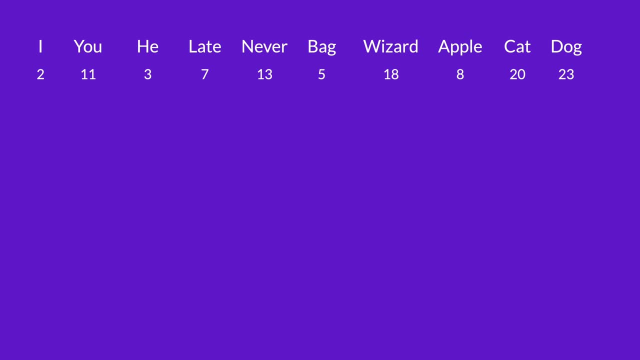 correspond to these numbers if you represent them in the embedding space. this is what you would have, and the distance between these two points would give you the similarity between these two data points. instead, if you embed your data to two values, you can represent them in a two-dimensional space. 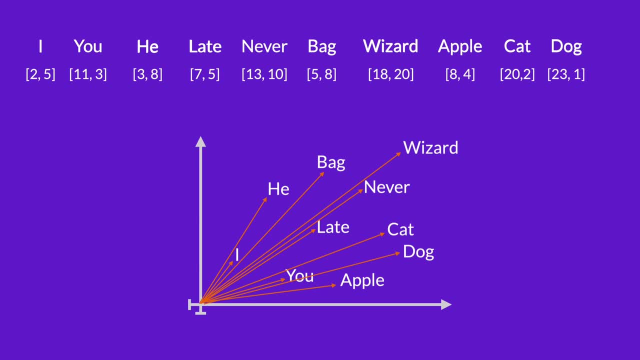 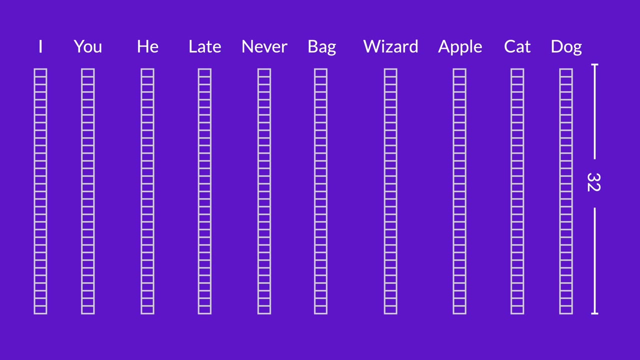 and now they will look like vectors with the direction only after the third dimension. we will have some issues visualizing the vectors, but they follow a similar logic. so if we embed a word into a vector of length 32, this means we are turning it into a vector in a 32 dimensional space. we cannot. 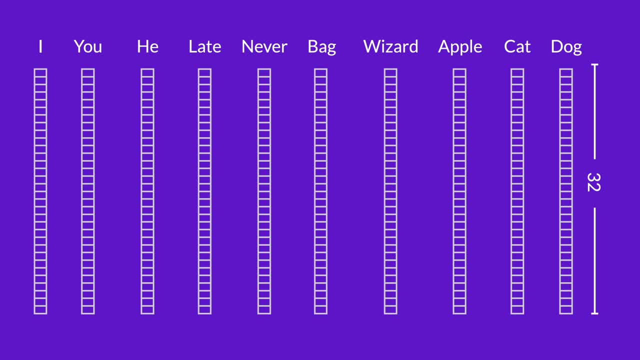 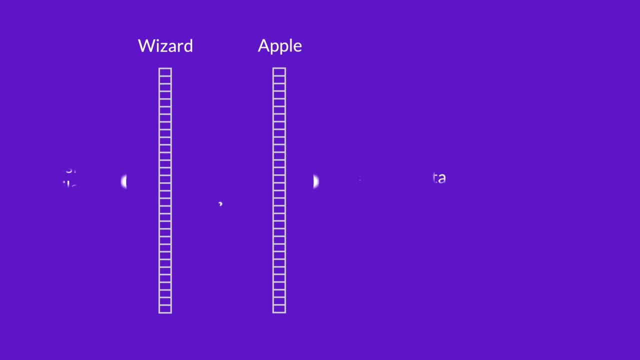 visualize it anymore, of course, but we can still calculate the distance of two different vectors or embeddings to each other, like we did with the one-dimensional example, by using things like cosine similarity. here is what we would want the embedding space to look like if we trained a 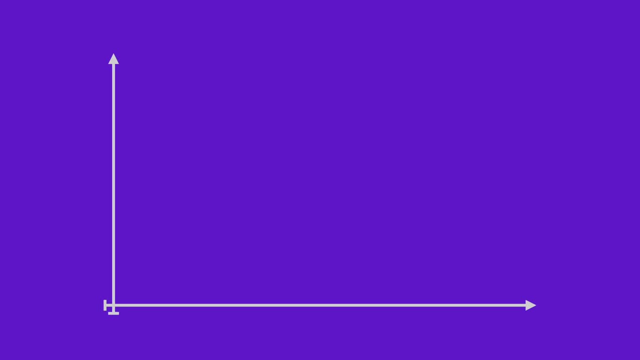 successful word: embedding. since we cannot visualize 32 dimensional space, let's use this representative 2d space. in this embedding space, we want similar words to be closer to each other, for example king, queen, sovereign kingdom or another group could be cat, dog, pet, bird, animal, for some. 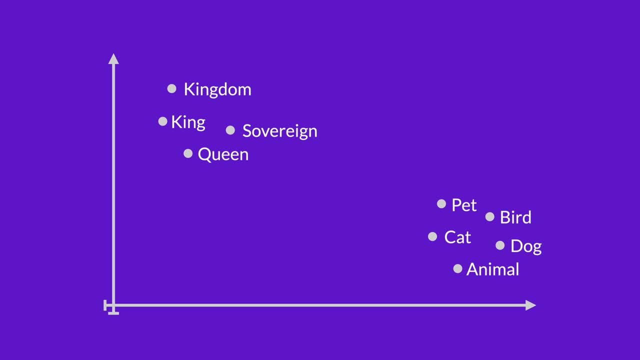 cases it is even possible to make sure that the relative distances between words represent contextual information. in a very commonly used example, if this is how a man and woman are positioned, related to each other, this is how king and queen would be related. so by subtracting the vector for man from the vector for king and by adding woman vector to it, you 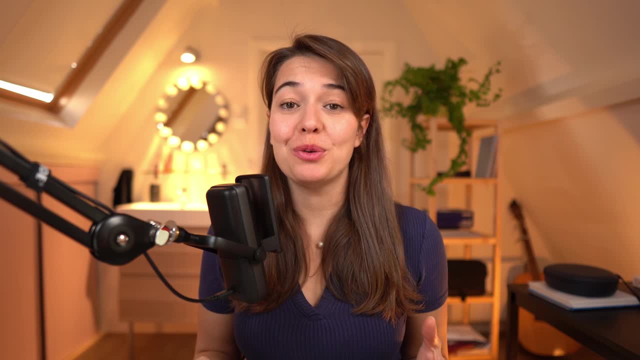 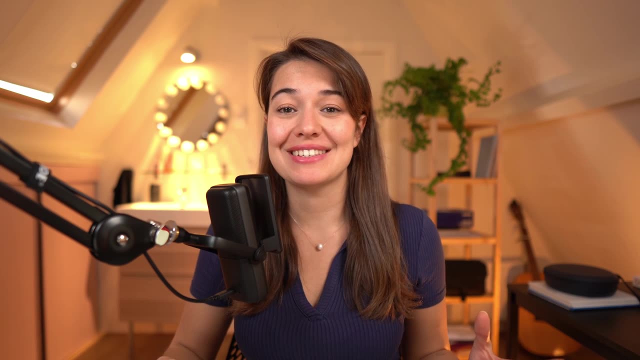 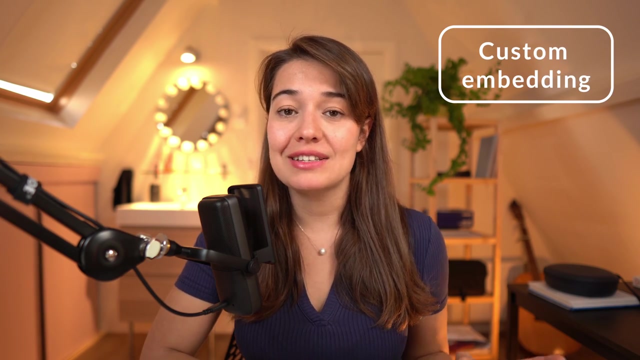 get the vector for queen. okay, so this has been cool, but how are they made? word embeddings are made in the same way, so let's look at these two methods. one is the code that you learned from big corpora. that is basically just a lot of text. there are a bunch of different approaches to how. 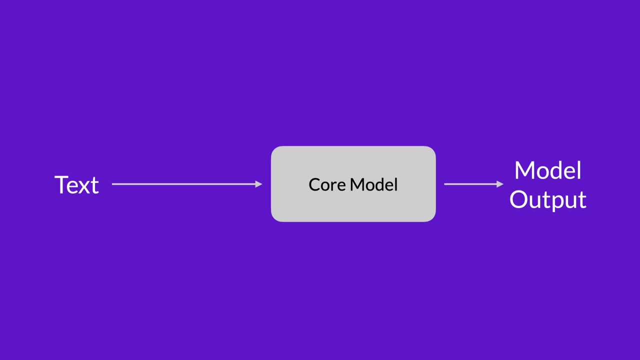 to make this happen. so let's look into that now. one thing you can do is to have a custom embedding layer in your model. so what you need to do is let's say: this is the core of your model, where the actual learning happens. before you feed the text to your model, you can have an embedding 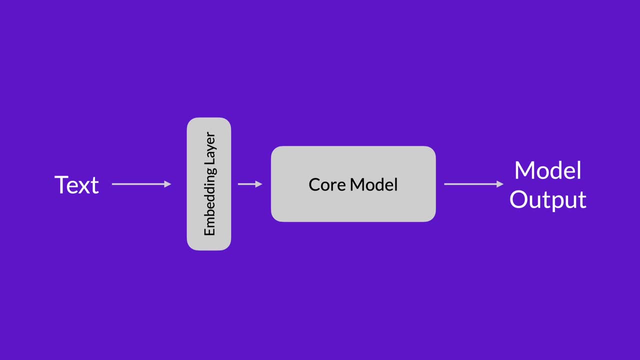 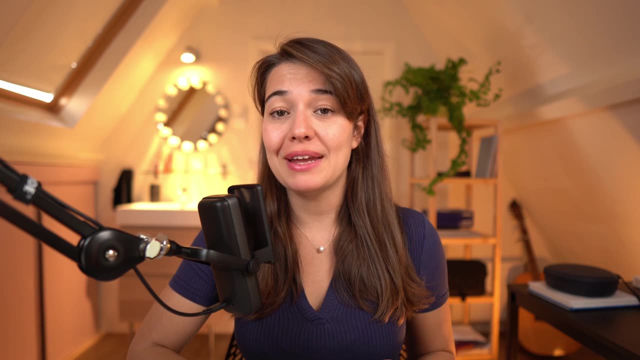 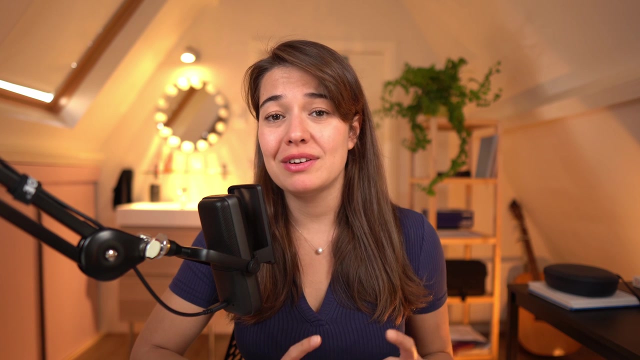 layer and just initialize it with random weights and parameters, and then you can also create your own embedding layer, which is all about both the code and the numbers and the number of words that you think is right and the color. so it's almost a very basic example of how to represent the words in the best way. the advantage when you do it this way is: 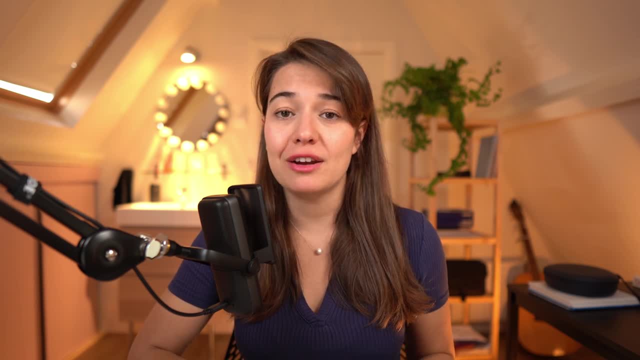 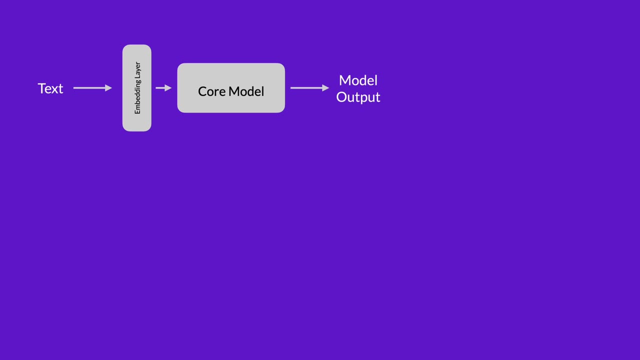 that you will have an embedding that is very specific to your use case and it will be specialized to your data set. but the problem is, to have a very successful and well performing embedding layer, you would need to train it with a lot of data and it will probably take a long time. 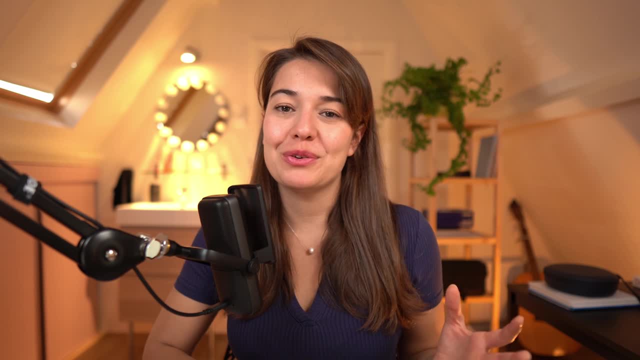 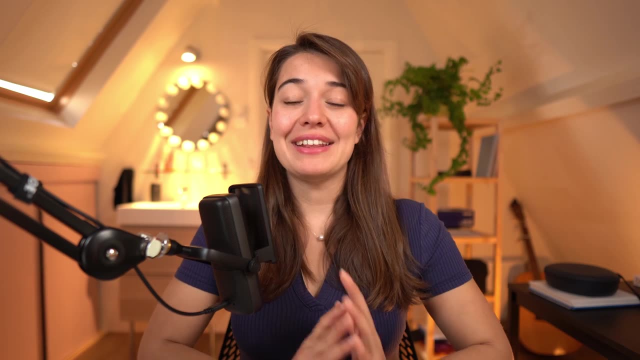 take text and turn it into numbers. if you would like to learn more about the transformer architecture and how that model works, you can go and check out our video on transformers. another approach is word2vec. word2vec works by getting the one hot encoded versions of the words. 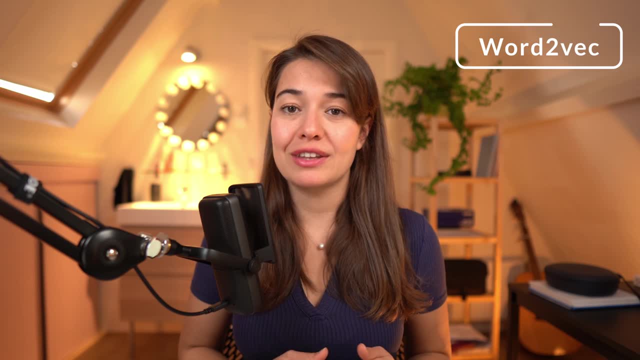 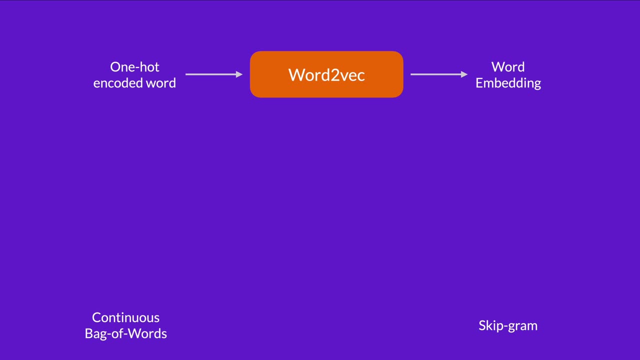 and creates embeddings of these words by using the context of the sentence too. there are two different approaches to word2vec. one of them is called continuous bag of words and the other one is called skipgram. so here's how it works. given a corpus of text, so a lot of sentences, what we do is: 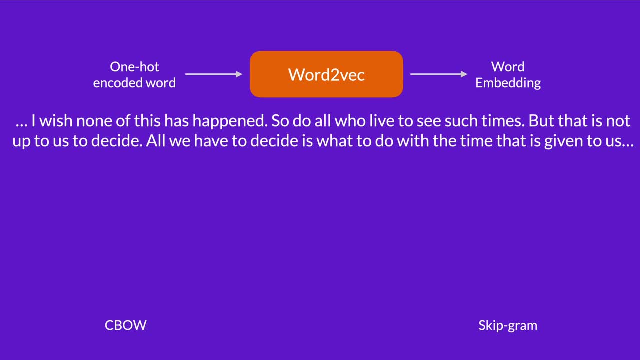 we divide these sentences into groups of n words, so for the sake of this example, let's say three. so in this sentence we take three words with c, both or continuous bag of words. we take the two words surrounding the middle word and we feed it to a neural network and we try to 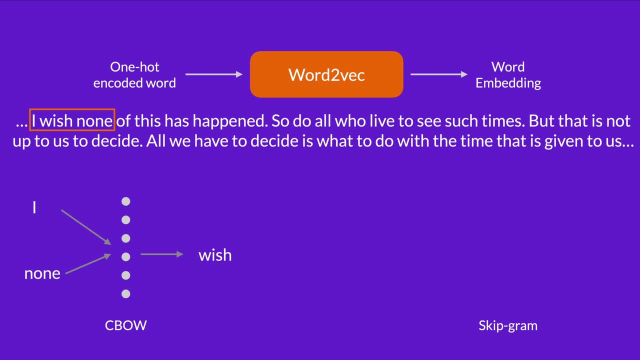 guess the word that should be in the middle, whereas for skipgram we do the exact opposite: we take the middle word and we try to guess the words that should be surrounding this word. we keep training this model by sliding this window to the right every time. in this model, the neural 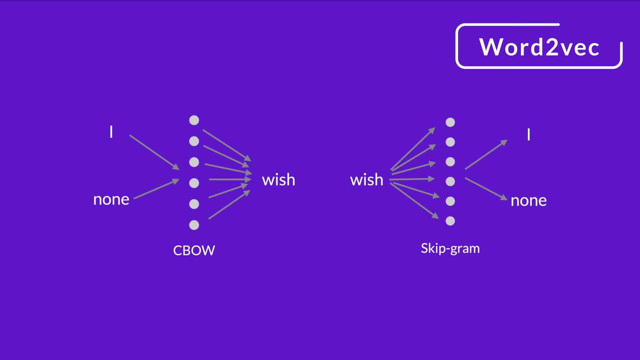 network only has one layer, so only one hidden layer, and the number of neurons in this hidden layer is the size of the embedding. once the network has good performance, we can extract the embeddings of words from this network. for SIBO, these are the output weights and for skipgram, 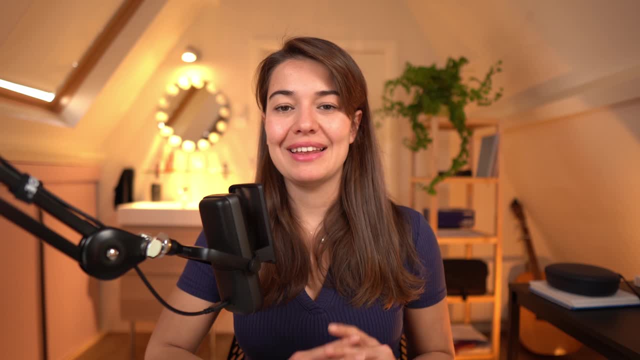 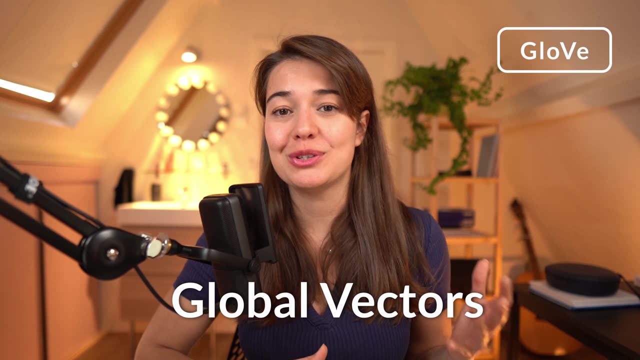 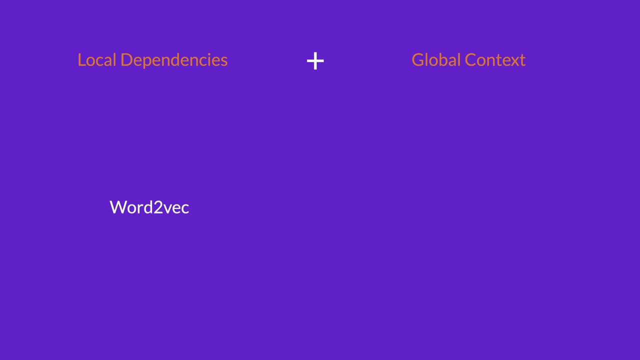 these are the incoming weights corresponding to a word. next, we have glove. glove stands for global vectors and it is an extension of the approach that we've just seen, word2vec. it is an extension of word2vec because it not only looks at the local dependencies of words, but it also looks at the global context of the whole sentence. 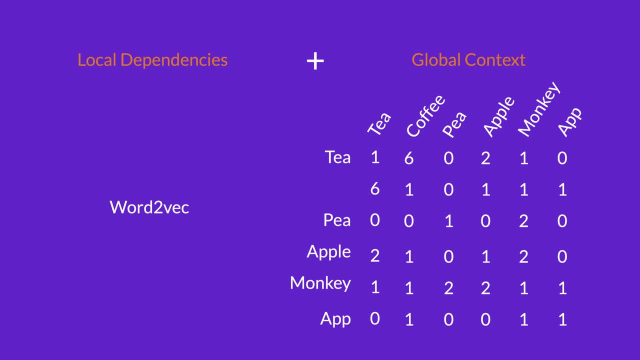 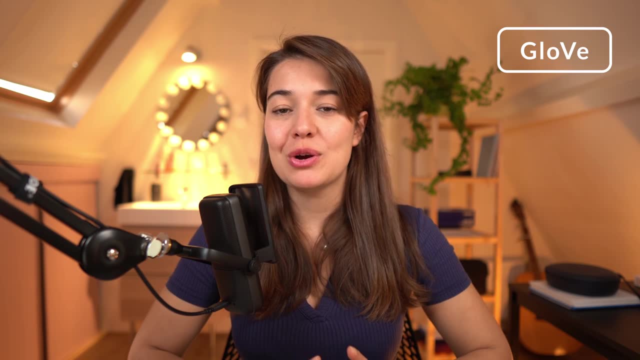 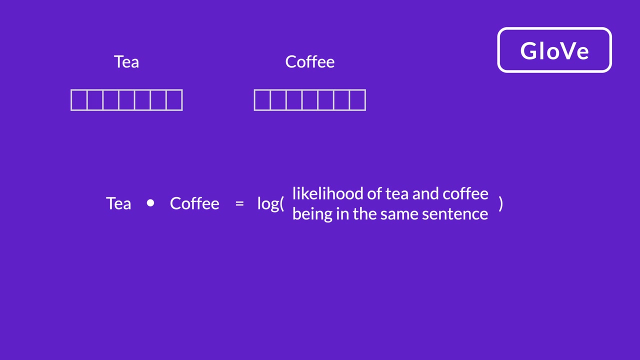 it does that by taking into consideration the co-occurrence metrics of the sentence. the training principle of glove is a little bit too complicated to get into in this video, but all you need to know is that the training objective of glove is to learn word vectors such that their dot products equals to the logarithm. 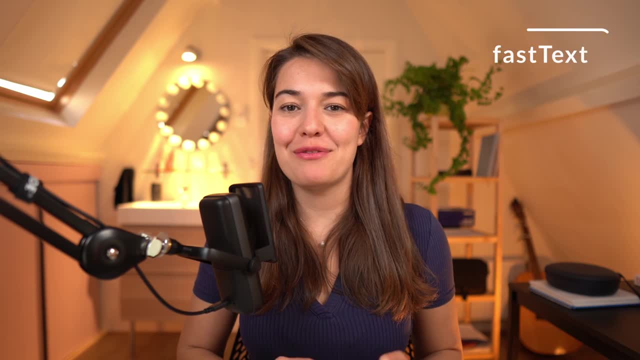 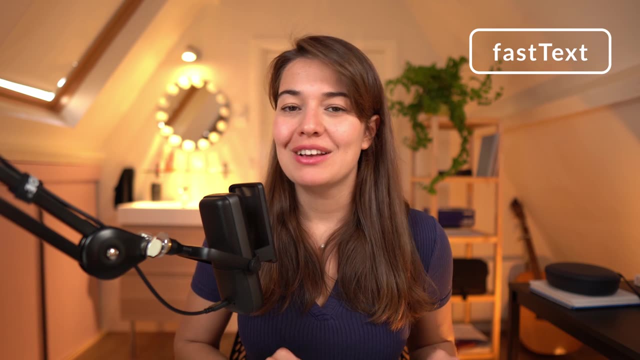 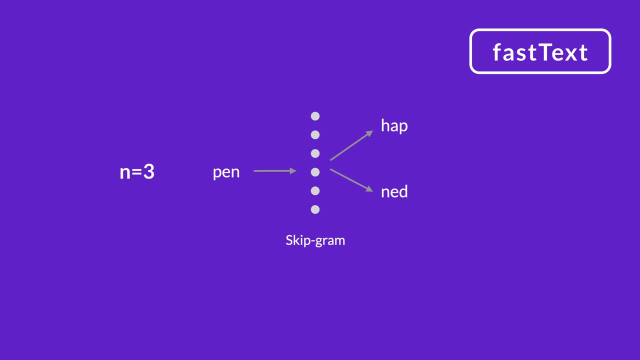 of the words: probability of co-occurrence. next we have fast text. fast text again is an extension on the word2vec algorithm, but this time in a bit of a different way. so instead of taking a skipgram model and training it on whole words, what it does is to separate these words into subwords of length. 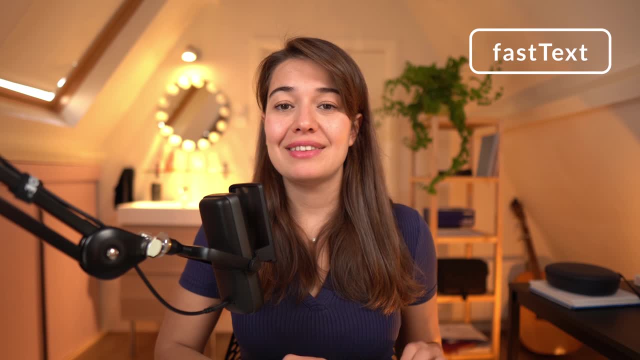 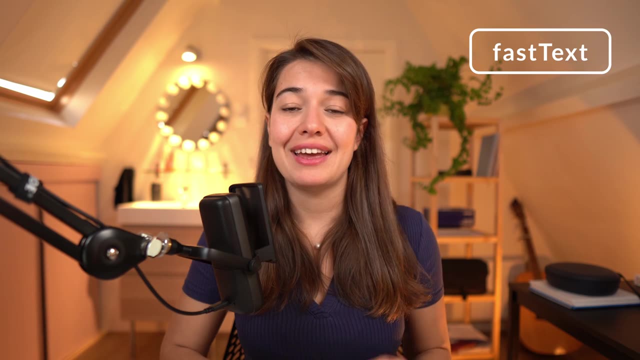 n and train the model on top of these subwords. thanks to the subwords approach, it works really with rare words or words that were not seen in the training data, and this is honestly a huge advantage of fast text over the previous ones we saw. another advantage of using subwords is that 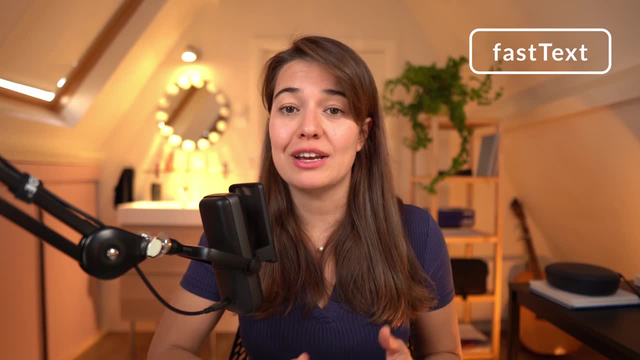 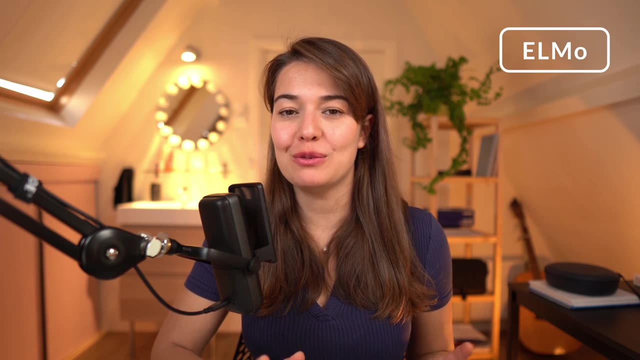 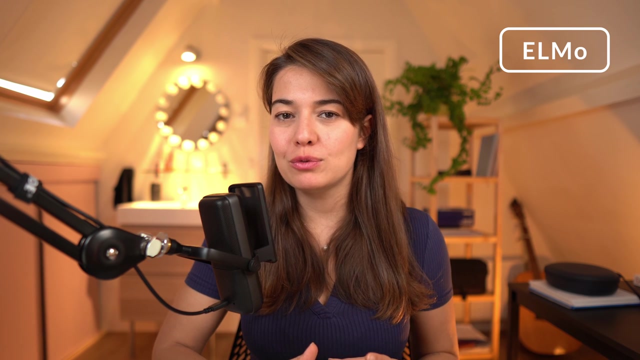 it does really well with morphologically rich languages like german or turkish. and lastly, we have elmo. elmo is one of the latest innovations in the area of word embeddings. with elmo, the embedding of the word depends on its context, so in a way, the embedding of the word is created dynamically. 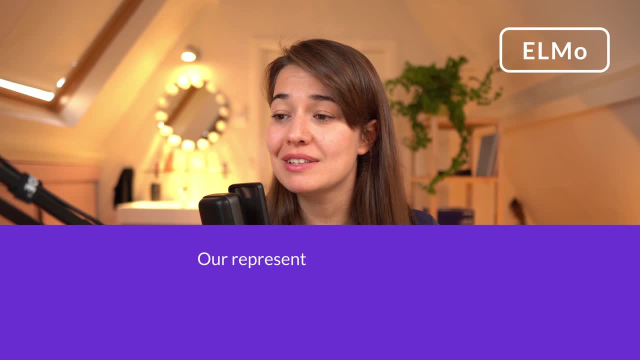 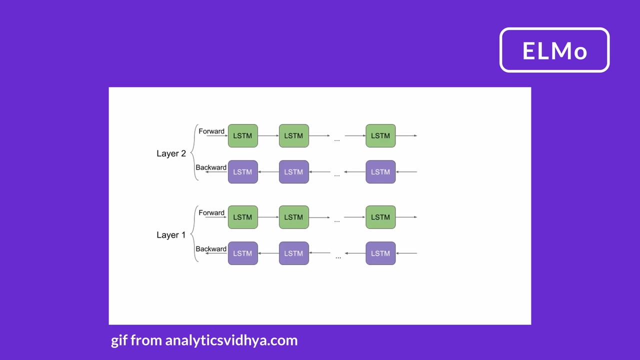 and the paper. they mention this by saying: our representations differ from traditional word embeddings in that each token is assigned a representation that is a function of the entire input sentence. elmo representations of words are derived from a bi-directional lstm model that is trained on a language model task of predicting the next and 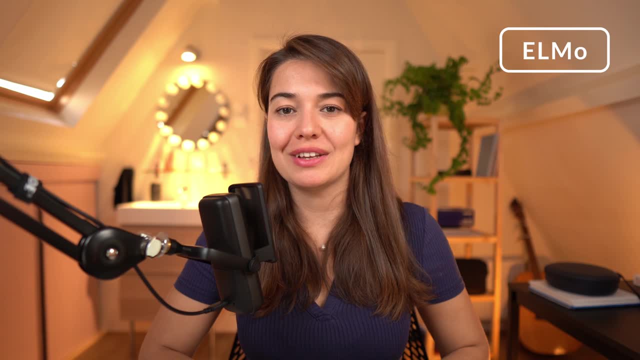 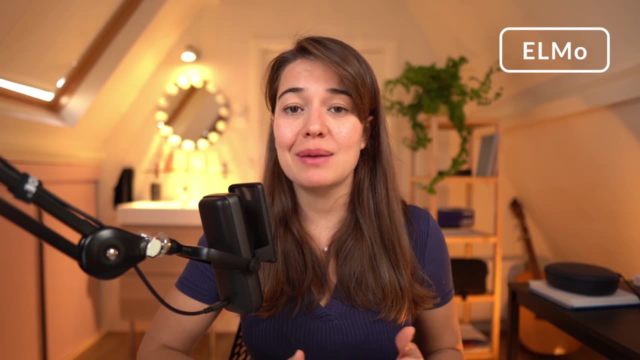 the previous words in a sentence. By training on a language modeling task, Elmo takes the context of the sentences into account while it's creating the embeddings, And this way it is able to distinguish homonyms of words, for example. So the embedding of the word fair would be different in these two. 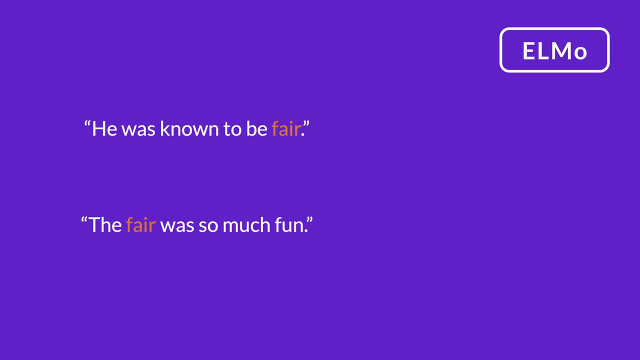 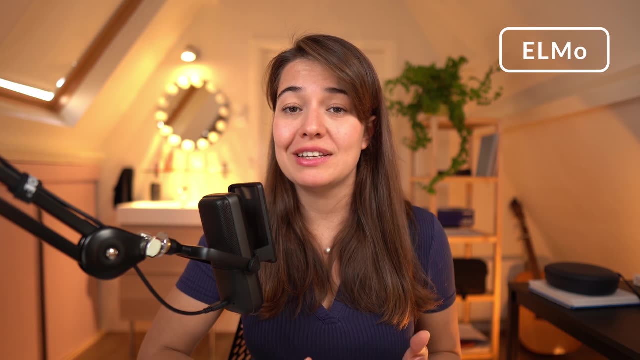 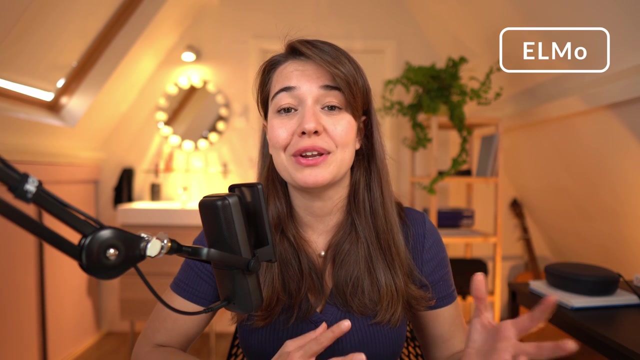 sentences. He was known to be fair. The fair was so much fun And because Elmo's first layer deals with characters instead of whole words, it is really good at dealing with misspelled words or typos. But all in all, Elmo needs its own video to explain to you fully what it does and how it. 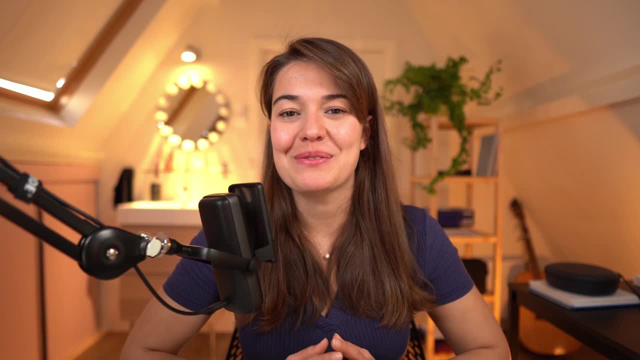 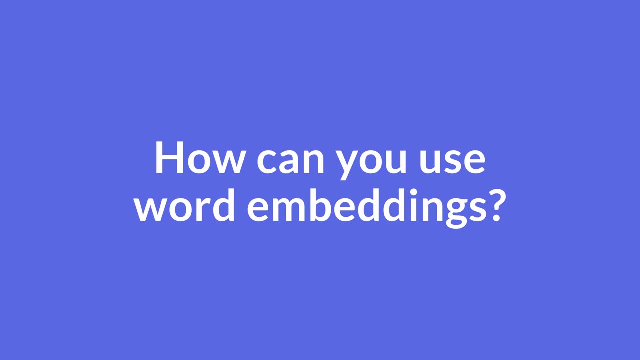 trains. If you want to see that video, leave a comment and let us know. Okay, so we've seen some cool ways of how word embeddings are made, but how can you use them in your project? So there are mainly two different ways. You can either make a word embedding yourself from scratch, or you can 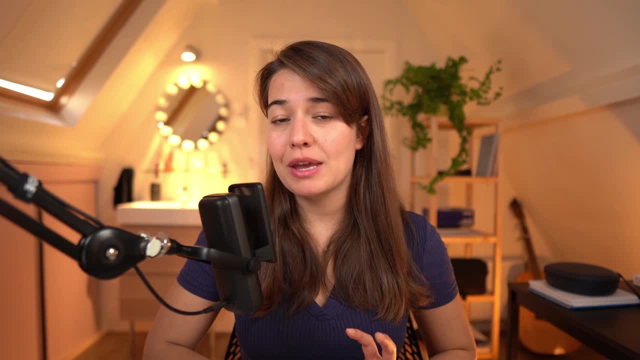 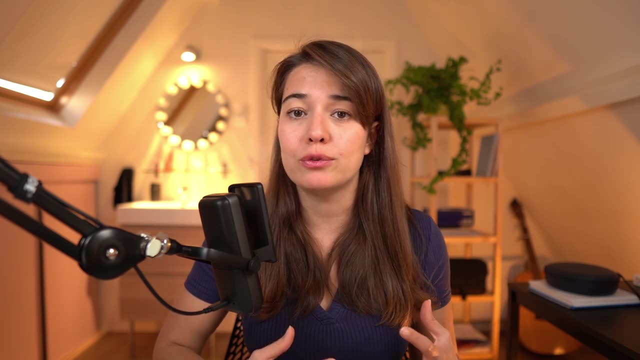 use pre-trained words. So if you want to learn how to make a word embedding yourself, you can use word embeddings. It is not that hard to make your own word embedding because for all of these algorithms and models that we talked about, there is a library that offers you a pre-made model that. 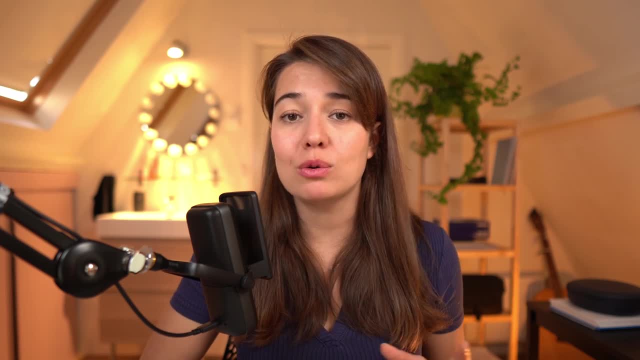 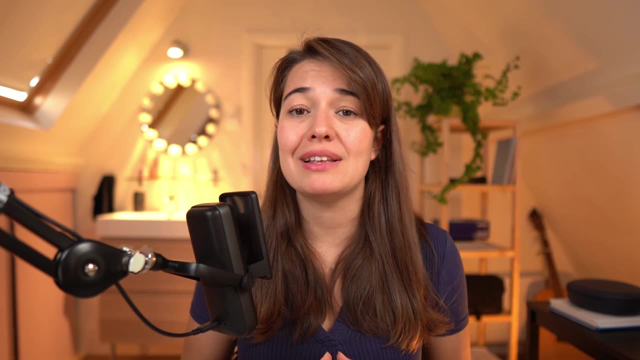 you just need to push data through. But the problem is- like we also mentioned in making an embedding layer by yourself- is that you need to have a lot of training data and it will probably take a very long time to achieve a good performance, But at the end you will have a word. 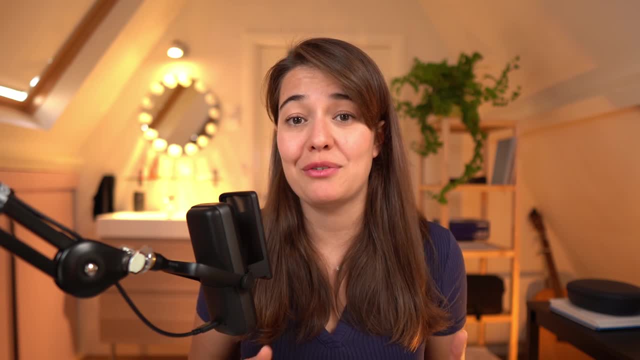 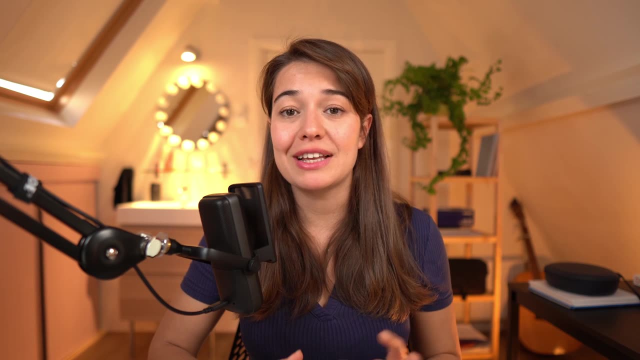 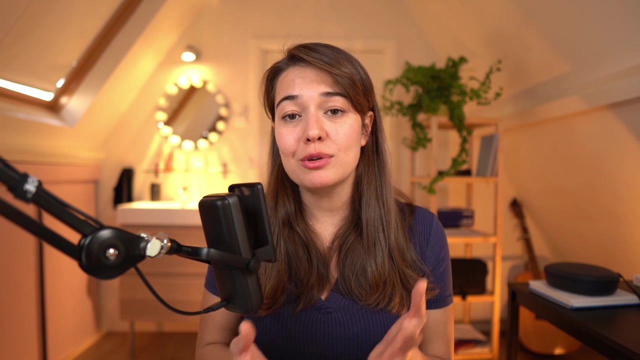 embedding that is specific to your use case and it will be very easy to use. So, if you want to use a pre-trained word embedding, there are libraries that offer pre-trained word embeddings and even the research groups that come out with the new ways of embedding words most of the time. 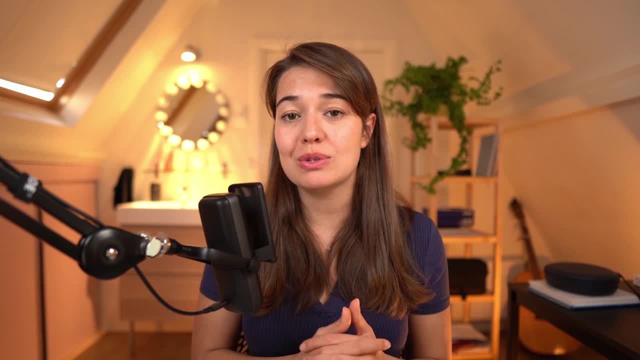 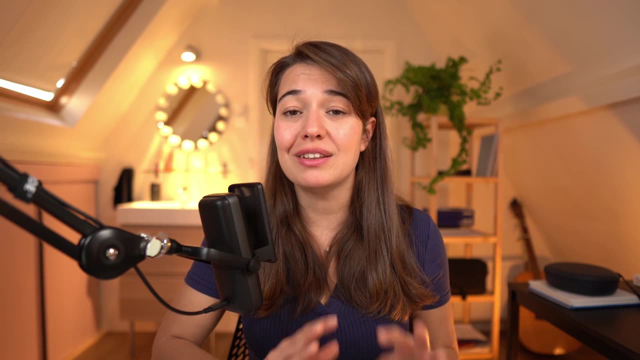 release their word embedding model to the public use. These word embeddings, of course, will not be specific to your use case, but at the end of the day, they will save you a lot of time and effort. There are two ways how you can use those pre-trained word embeddings. 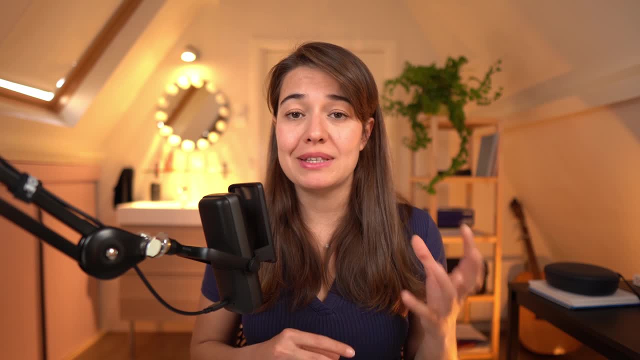 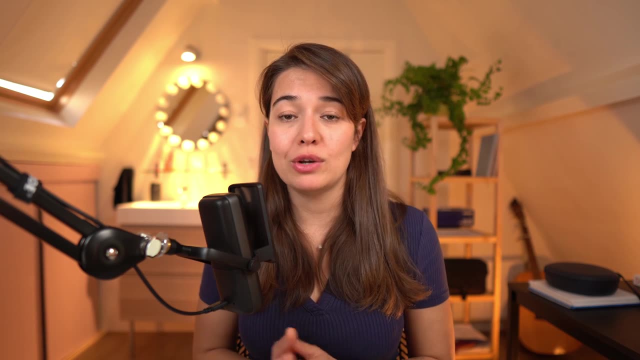 Depending on the embedding that you're using. you can either use them statically, so not update them during your training, just kind of plug and play, or you can also make them part of your training process and kind of fine-tune them as you're training your model. Before we wrap up: 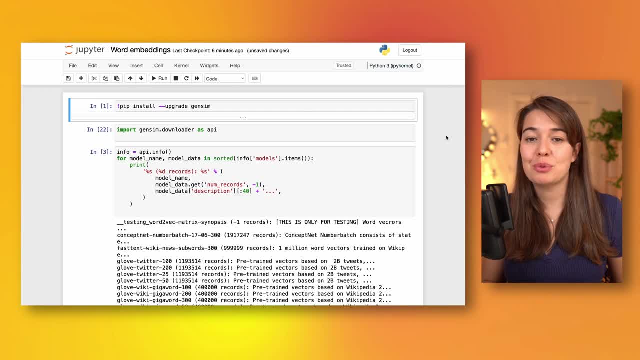 I want to show you how to import pre-trained word embeddings from the GenZoom library, because I think it's quite cool to see how they work and also kind of poke around a little bit. So the first thing that you need to do, of course, is to install the library. You can find more. 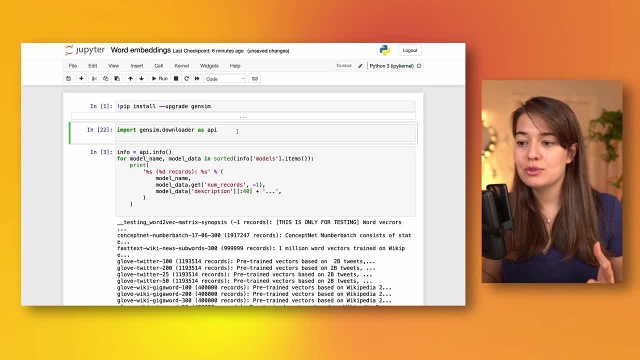 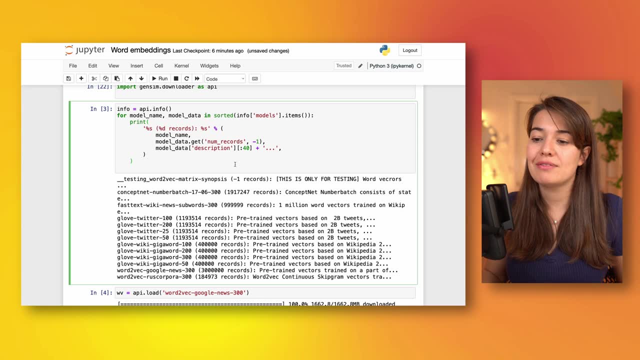 detailed instructions on how to do that on their website. of course, After we import the library, the first thing I want to look at is different types of word embeddings. pre-trained word embeddings they have And you can see immediately. they have FastText, GloVe and Word2Vec And even 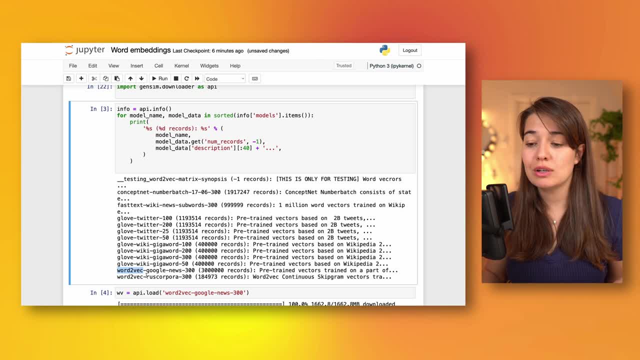 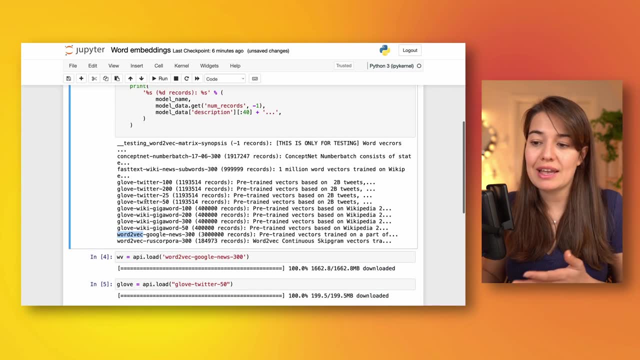 for GloVe and Word2Vec. they have word embeddings- pre-trained word embeddings that are trained on different types of data. You can read more about what kind of data they use, etc. there, but you can see they have Twitter data, Wikipedia data and Google News, for example. So 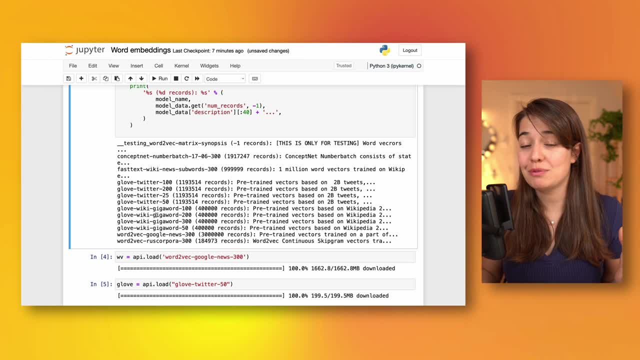 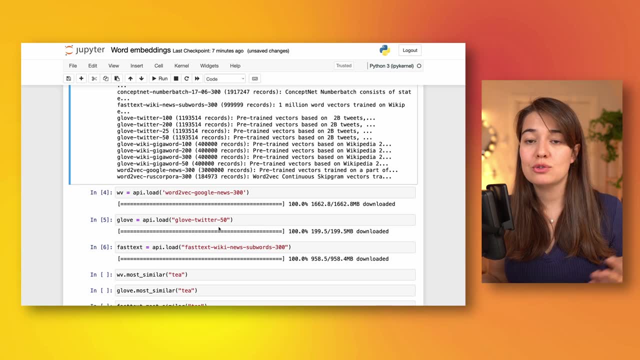 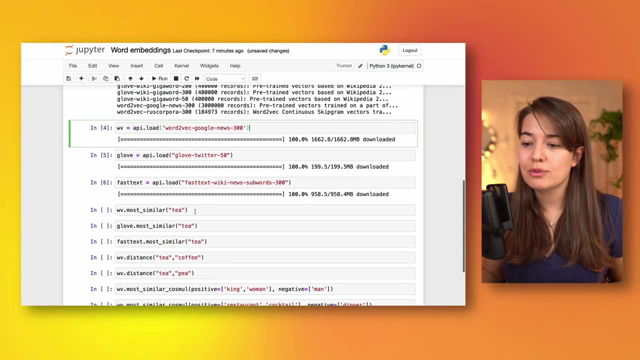 it's kind of cool. You can try and see which one works better for your specific project, And then I install or load these different types of word embeddings to my project And I would like to show you kind of the details of them and how to kind of poke around. So 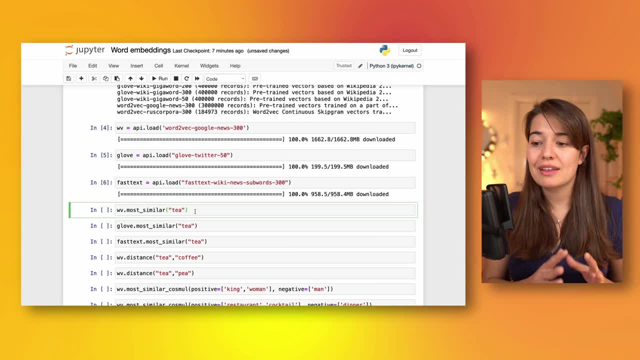 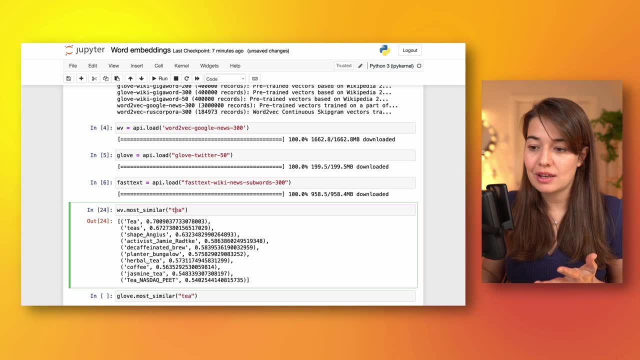 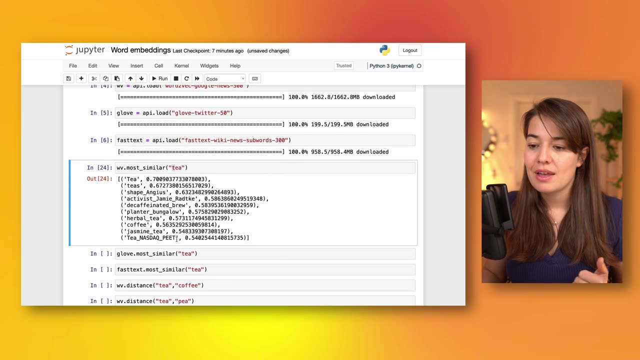 the first thing that I want to see is what Word2Vec thinks is the closest thing to T And it thinks it is. well, I wrote it with lower letters. it thinks it's T with the capital letter, T's and some other things that I do not fully recognize. But if I try the same, 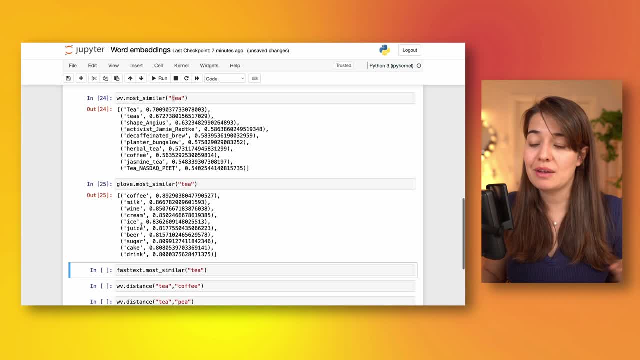 thing with GloVe. for example, it says coffee, milk, wine, cream, which is actually quite accurate. It's quite good. It thinks that the closest things to T are coffee, milk, wine, cream, ice juice, etc. These are all beverages or they have something to do with T, so that's quite good. 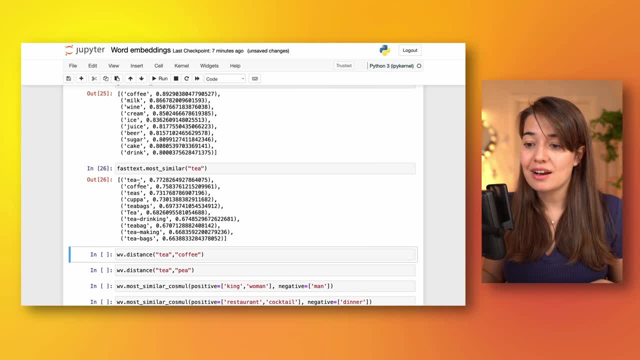 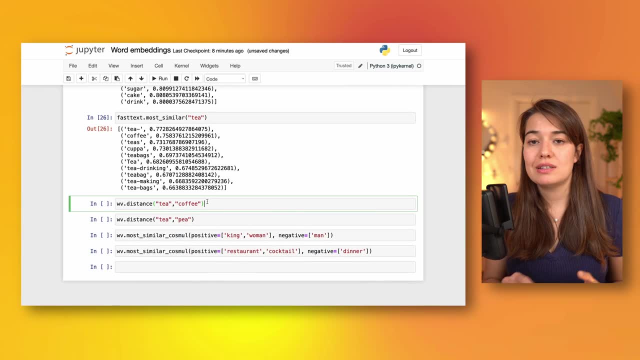 If you try the same thing with FastText, it again says T coffee, T's cuppa, T-backs- again, quite acceptable. You can also see the distance between two different terms. So, for example, if I like the example I gave in the video, if you look at the distance, 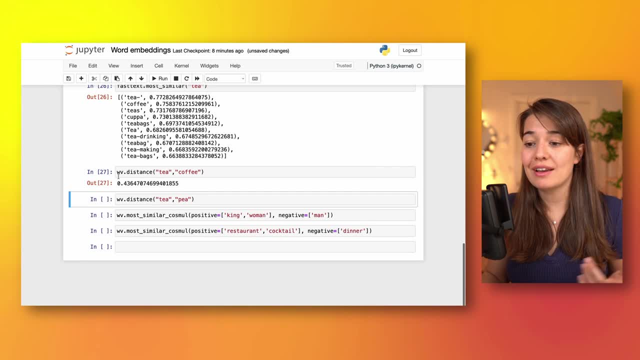 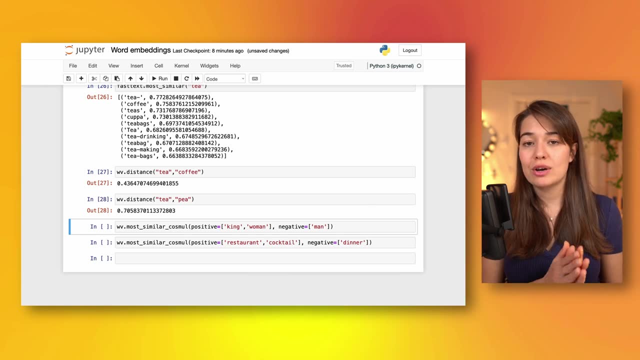 between T and coffee. it comes down to, for Word2Vec, 0.43,, whereas the distance between T and P is 0.7.. So that's quite good, As we said. what we want is that similar words are. 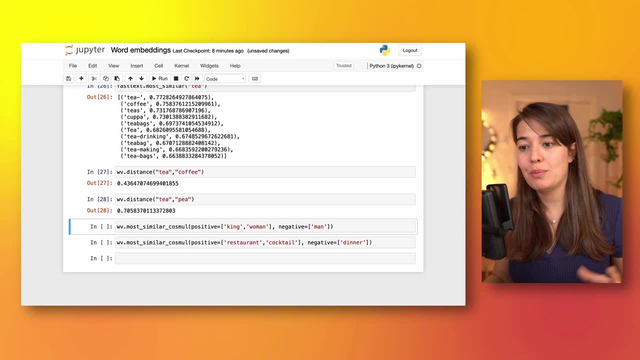 closer together and the words that are not that similar are farther apart, even if they are similar. So that's quite good. And then I would like to show you how to use this very similarly. Another thing you can do. another example that people use all over the 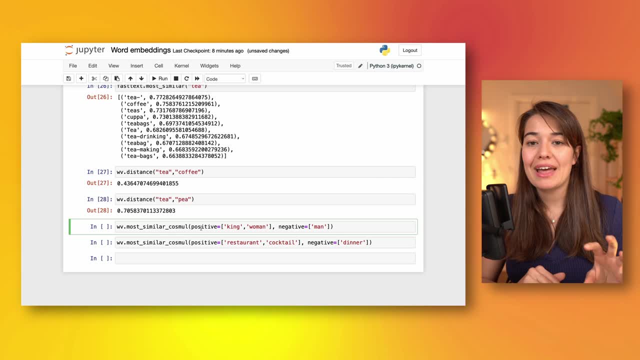 place is when you take the word king and then you subtract man from it and then you add woman to it, you want to arrive at a point to a vector that says queen, right. So here's what we can set that up. We say basically, positive is king and woman and negative is. 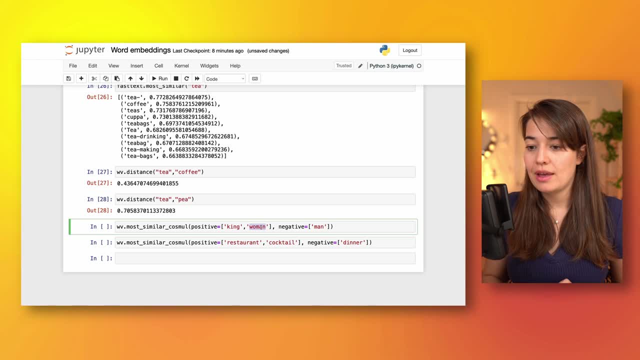 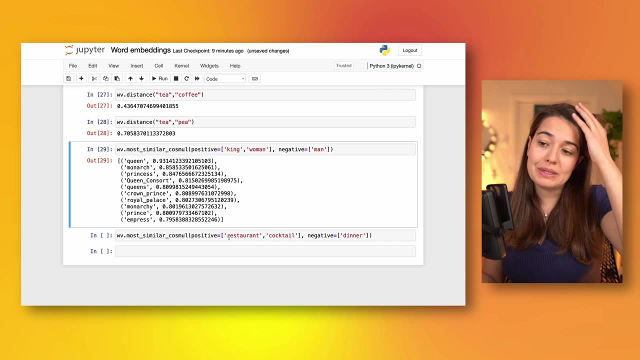 man. So basically, subtract man from king and add woman to it And we arrive at queen, and the closest thing is queen, which is amazing, And I wanted to. I mean, this is an example that is tried a lot, but I wanted to try something that I came up with. So I wanted to see if 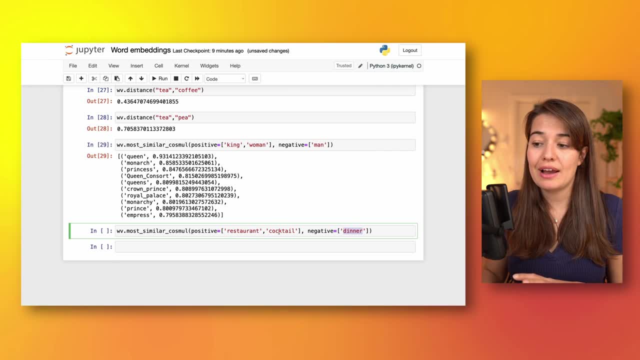 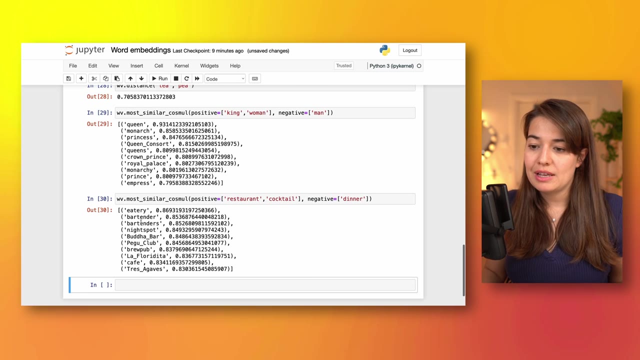 from the word restaurant. I subtract dinner and I add cocktail to it. I want to arrive at a place where you would drink a cocktail, so maybe a bar or something like that. So let's say, let's see what Word2Vec comes up with: Eatery, bartender, bartenders. 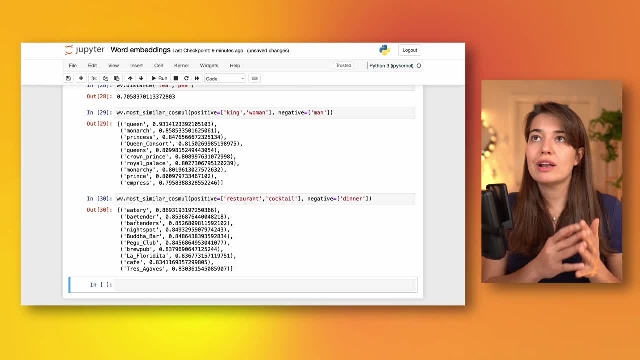 it is close enough. But of course you are not predetermining these relationships when you're making the word embeddings. Your word embedding model extracts these relationships from the text itself. So you know, of course you cannot always expect it to work perfectly. 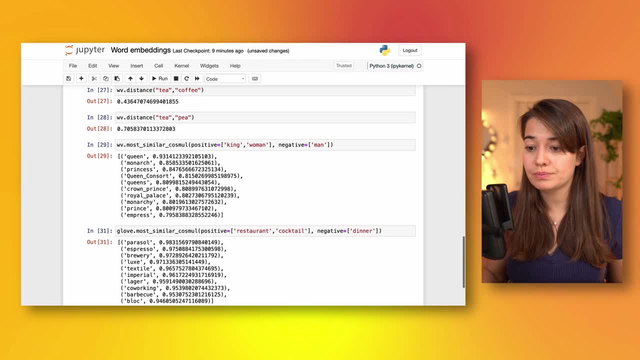 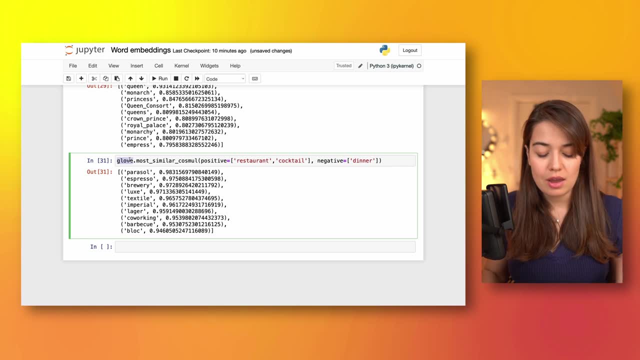 But I want to try it with Glove and see if it's better or worse Glove things. it's parasol espresso brewery- Again, not exactly what I was looking for, But maybe with fast text- Okay, this is a little bit better. It says bar restaurant.